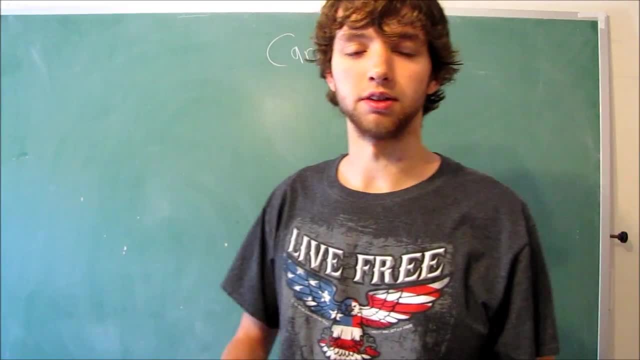 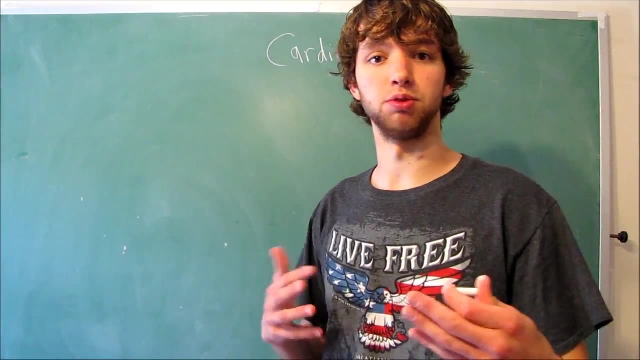 We actually talked about this a little bit, but we haven't really designed it or anything, because now we're talking about actually drawing out databases. Cardinality is basically the relationship type between a row of one table and rows or a row of another table. 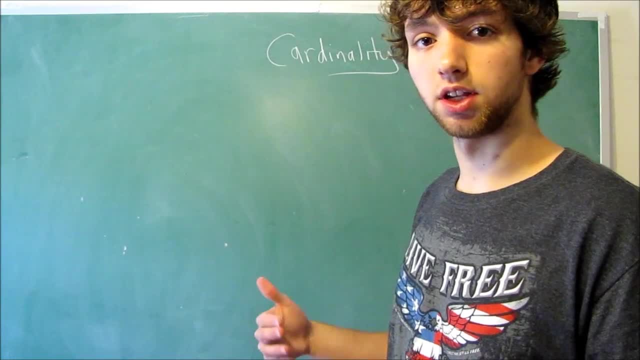 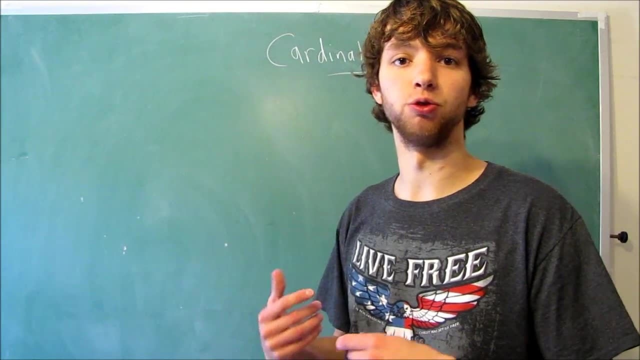 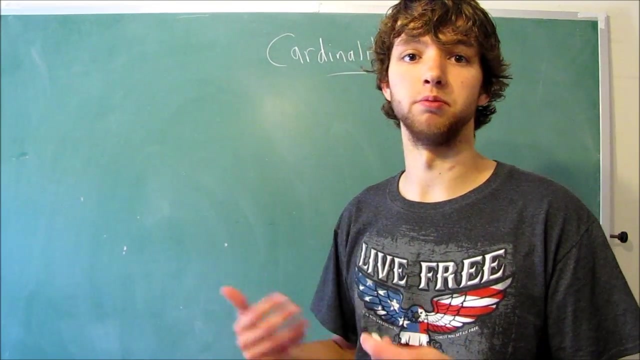 So the best example I have for this is a credit card database. So basically, a credit card company has a table for credit cards and then a table for cardholders, or the people who order the credit cards and use them to buy things. Basically, they're the credit card company's customers, I guess. 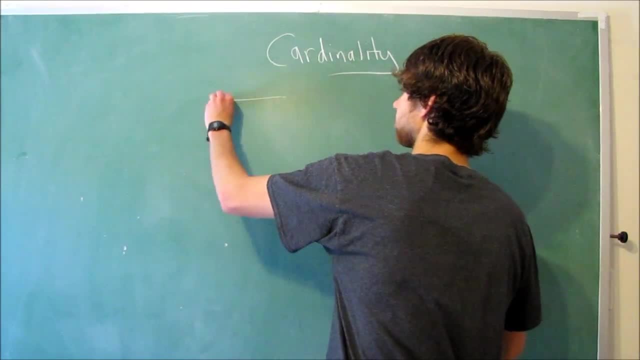 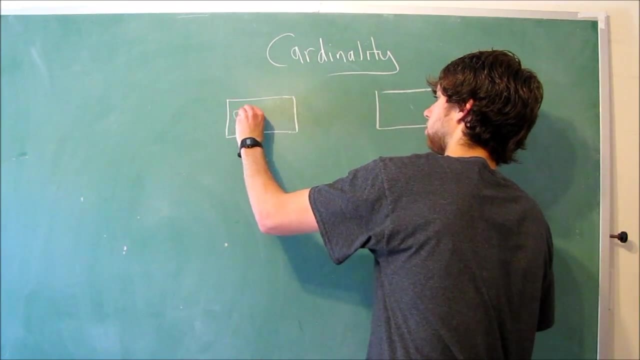 So I will draw those tables out, just so you can see this. I'm not going to draw them real big or anything, but just so you see How the connection works. So we have the cardholder And then over here we have the card. 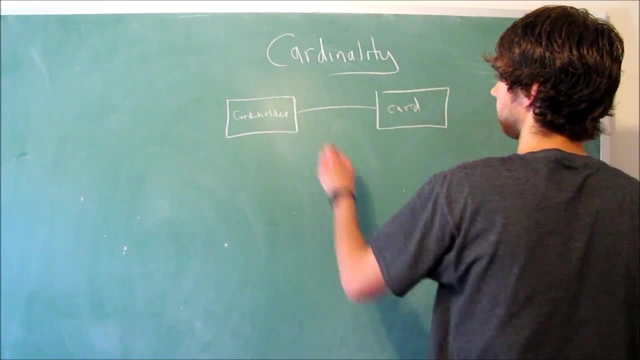 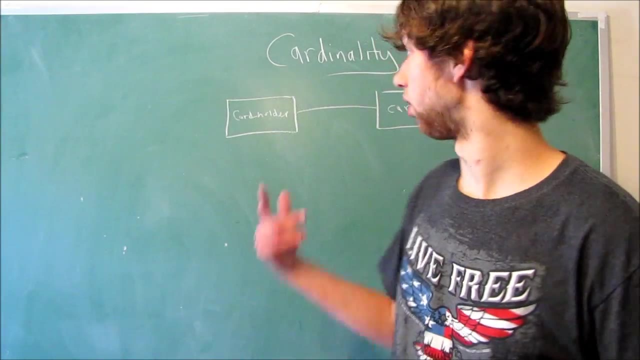 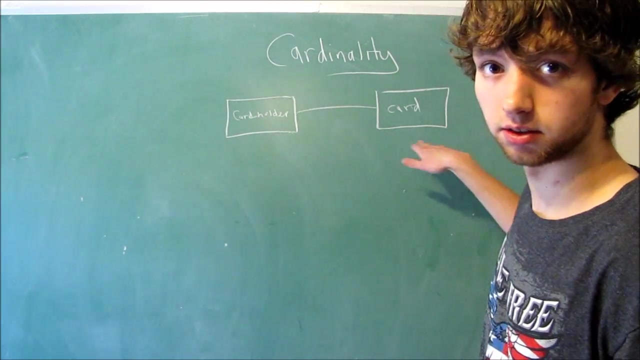 And there's some kind of relationship between here, between these two tables. Now, the only two possibilities for cardinality are one or many, Obviously for both sides, So you can have one to many, one to many or many to many. 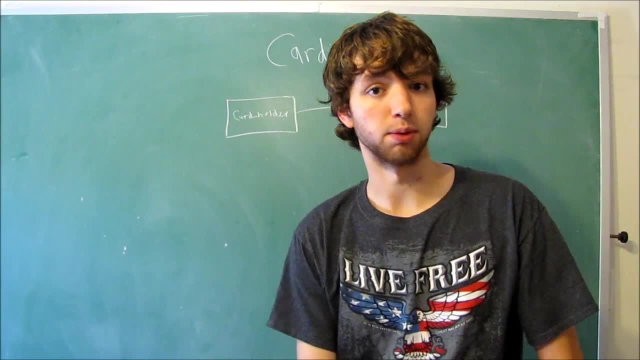 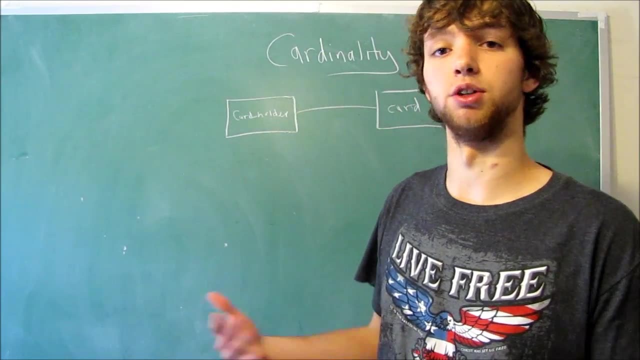 Those are the only three possibilities. Now, another thing to think about: when it comes to many-to-many. you might even consider that as not a possibility because you'd have to have an intermediary table, Which we talked about. that when we talked about designing many-to-many relationships. 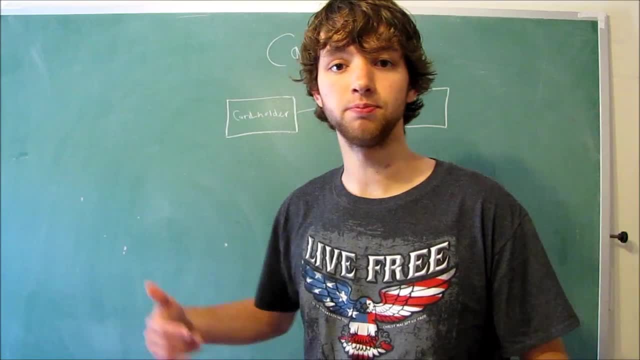 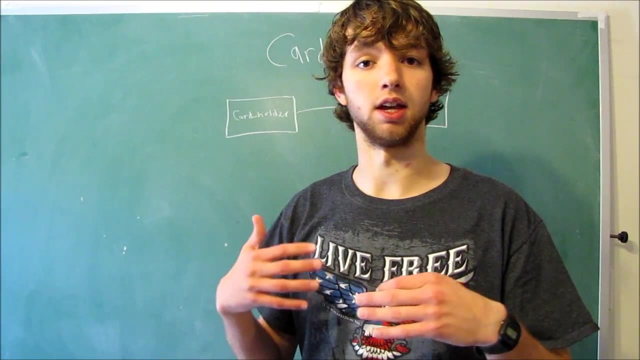 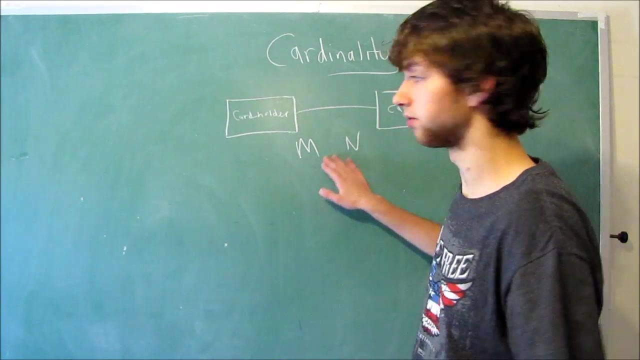 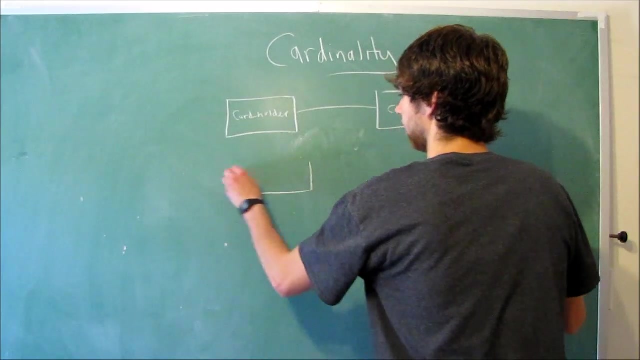 When we're talking about many-to-many relationships here, it's logical. What I mean by that is we're drawing it just like this And we would say many-to-many, And then when we actually implement that in a database, we would have to have a cardholder. 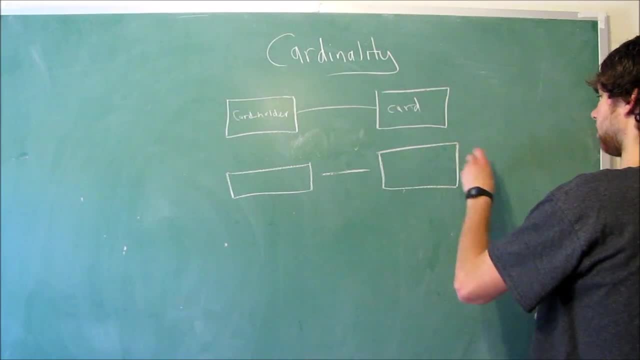 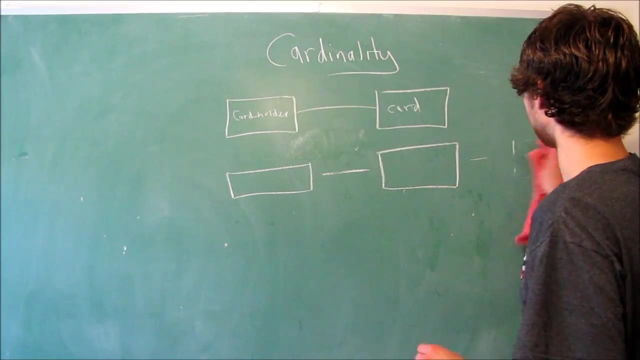 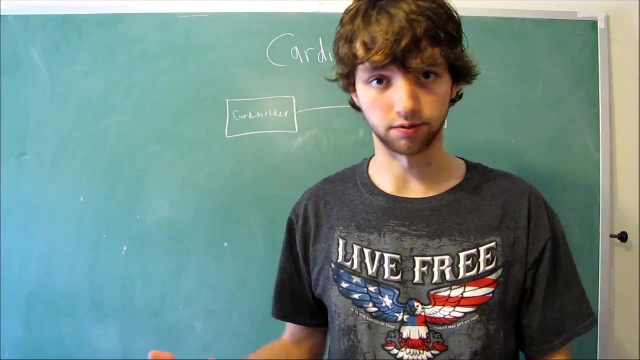 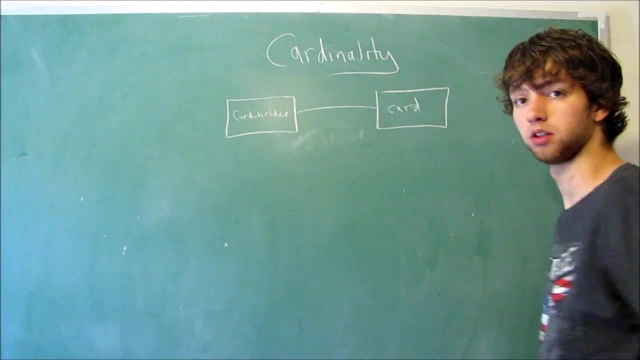 a cardholding table and then the cards table. That would be how to draw a many-to-many relationship. So hopefully that kind of makes sense for that. So in reality, when you're actually drawing out finalized products of databases, the only possibilities are one-to-many or one-to-many. 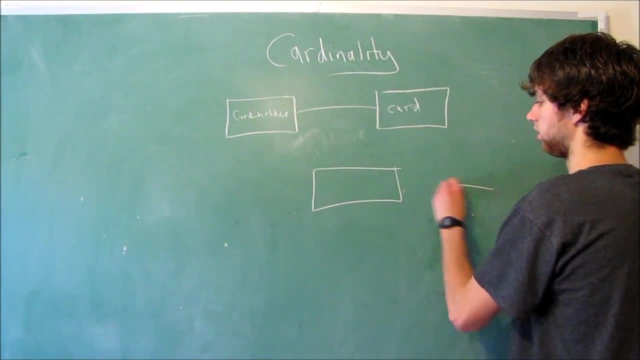 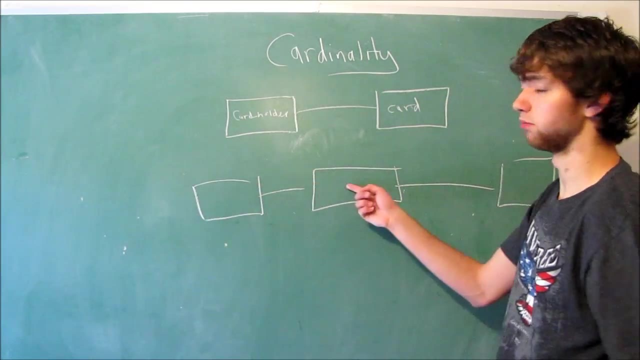 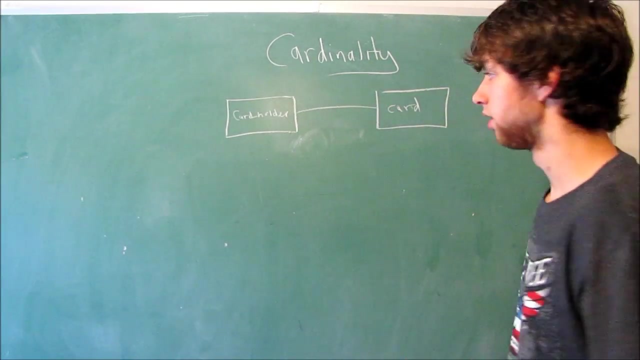 Because, even if you have an intermediary table, this is going to be a one-to-many relationship and then a one-to-many relationship, And there's a certain way to draw those out. That's what I'm going to be drawing right now. So a one-to-many. it's pretty simple. 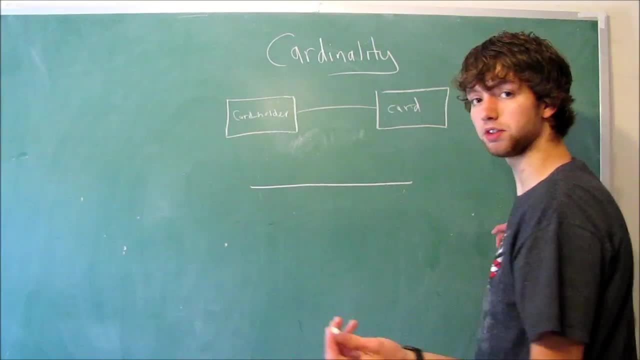 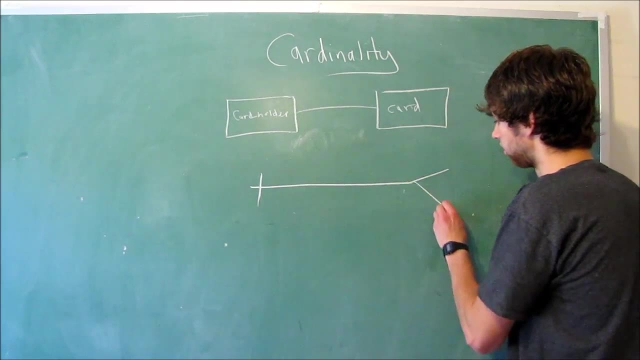 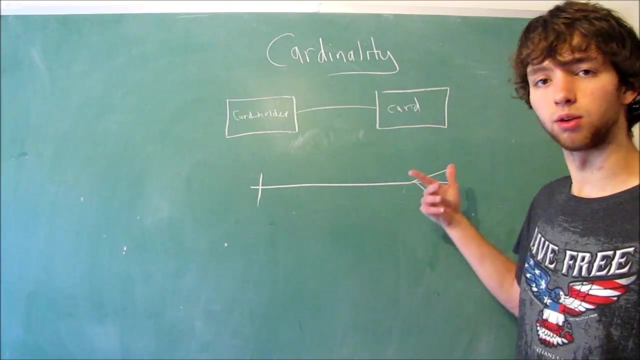 the one side, all you have is a straight up and down line like this. The many side you have this. This thing that we're doing right now is known as crow's foot notation, because it looks like crow's foot. 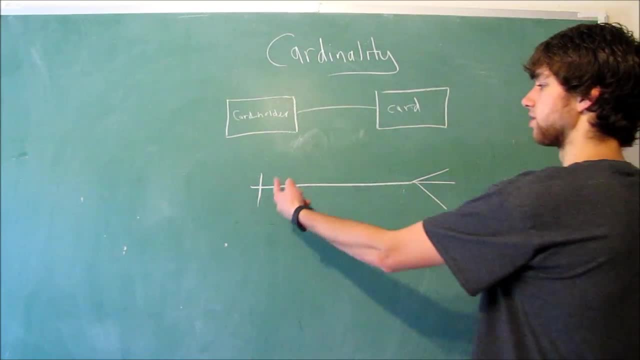 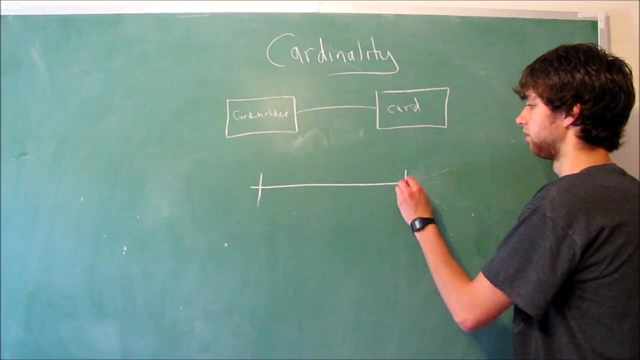 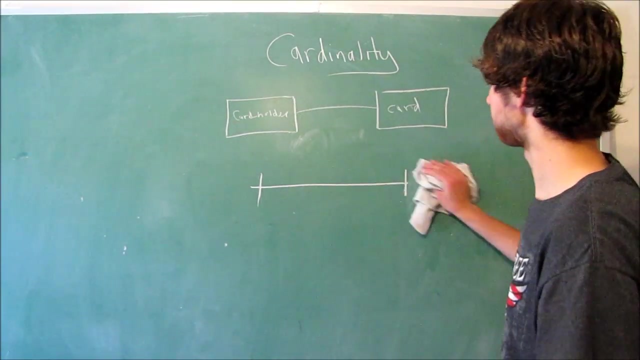 I think that's why they call it that. I don't really know. This is a 1.. This is a many, So when we're drawing it, one many, We could also have one-to-one, of course, possibility. I forgot to mention One to one Now, before we start drawing on both. 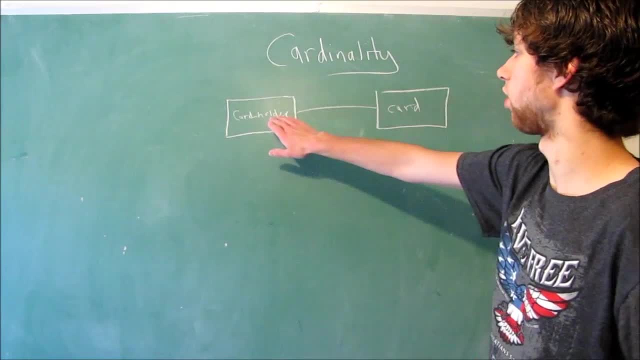 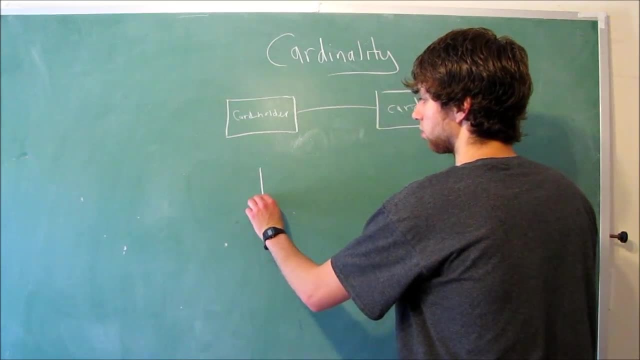 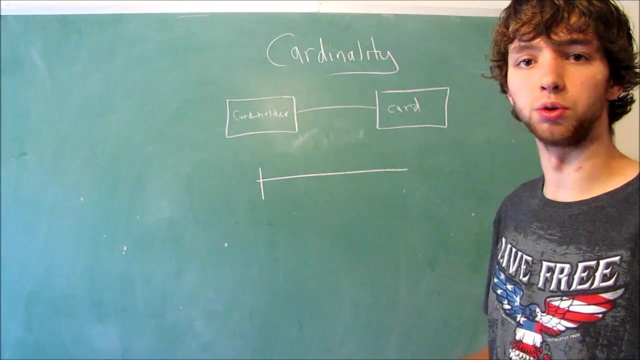 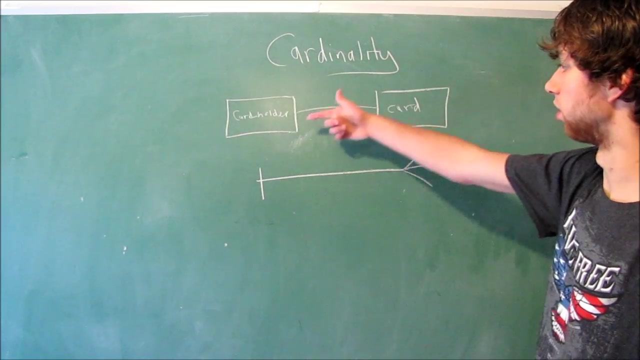 sides. I think it's easy just to think about one side. Think of a card holder relationship to a card. We would have one card holder. Now that we have that side figured out, we just think about the card holder. Then we can add in the card and we have many cards, So one card holder can have many. 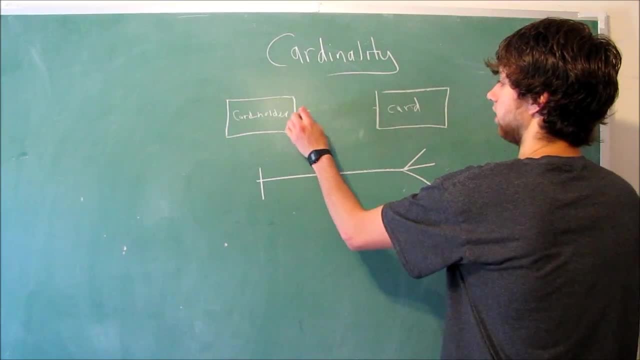 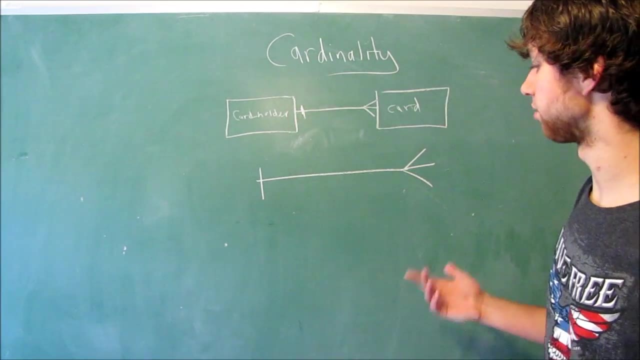 cards, and that's how you would design the line between the tables, like that. Now there's another thing we need to talk about, known as modality, which we'll talk about in the next video, but for this, we're just going to keep it simple. 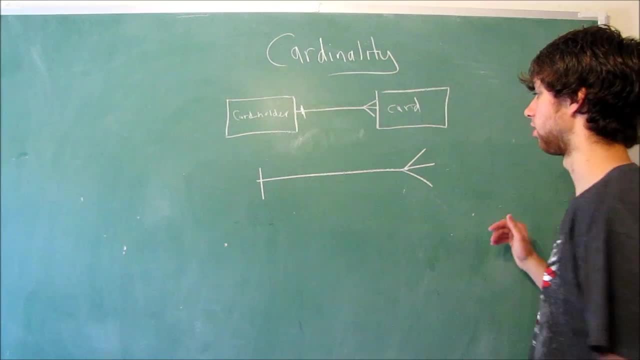 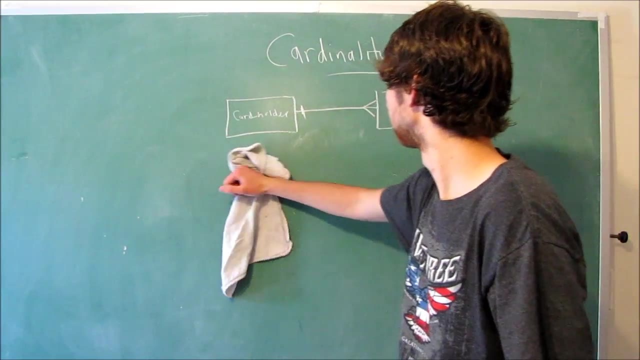 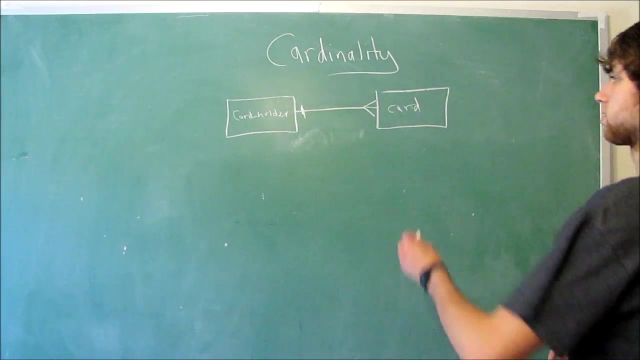 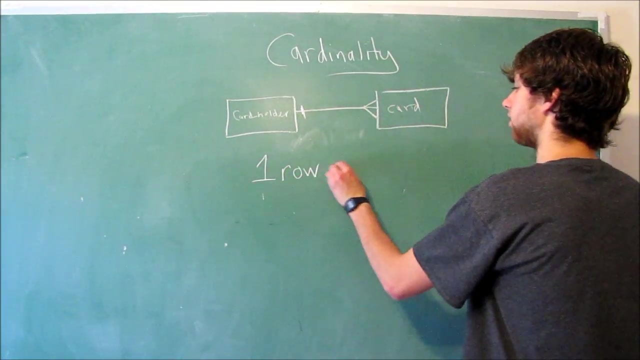 Just drawing these things here, but you might see also like circles. You might see a circle here, for example. We'll talk about that in the next video. So now you know how to draw a one-to-many relationship. So what does this exactly mean? That means one row can be connected with many rows in this. 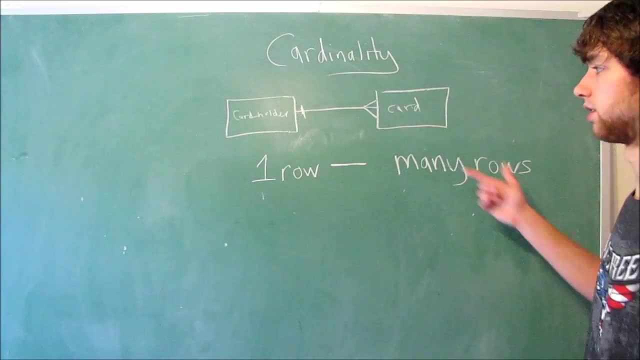 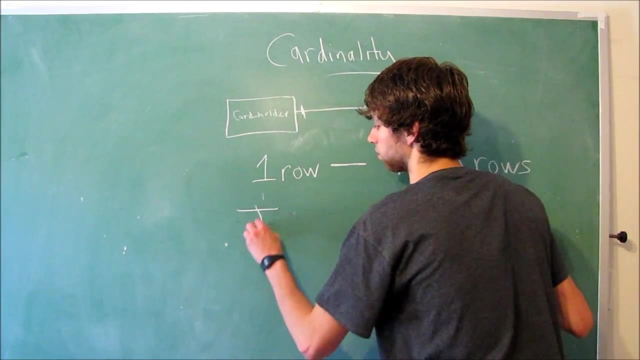 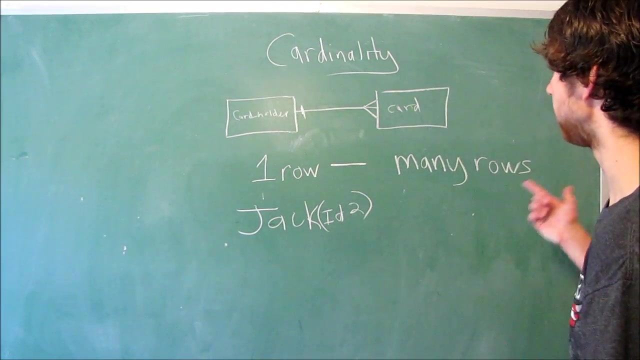 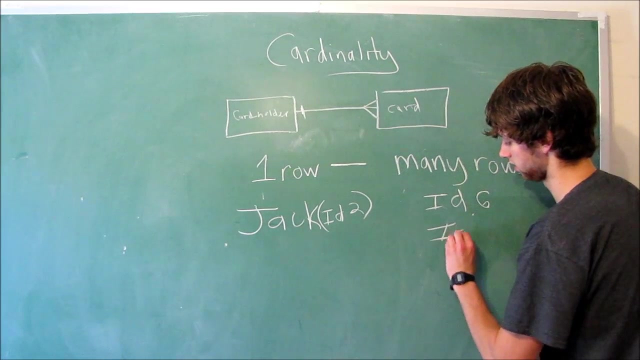 table. It's not necessarily the table, but the rows within the table. So we can think of a specific card holder. We can have a card holder with the name Jack, an ID of 2, and we can have many rows over here. cards: We can add a card with the ID of ID 6,, ID 8,, ID 12, and you can see. 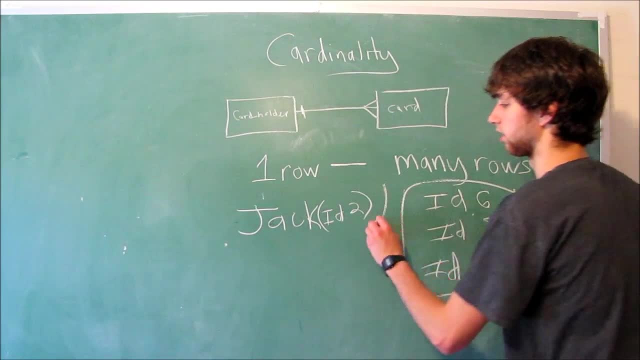 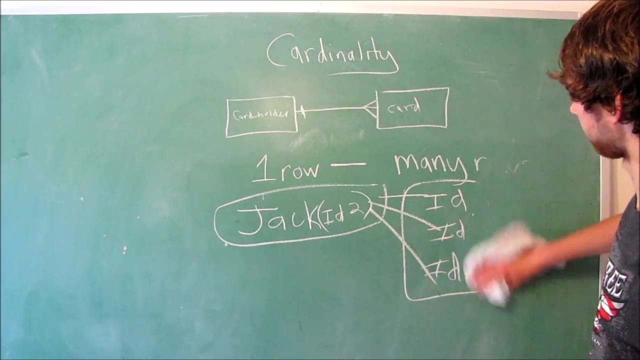 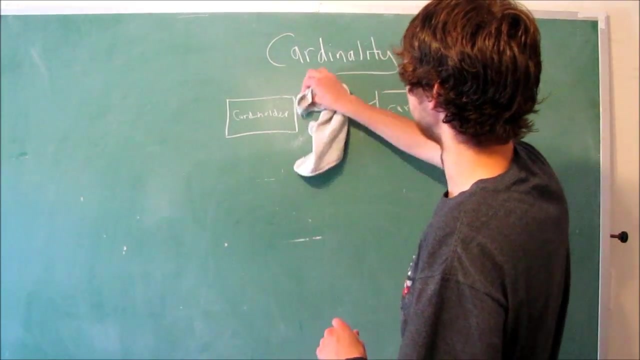 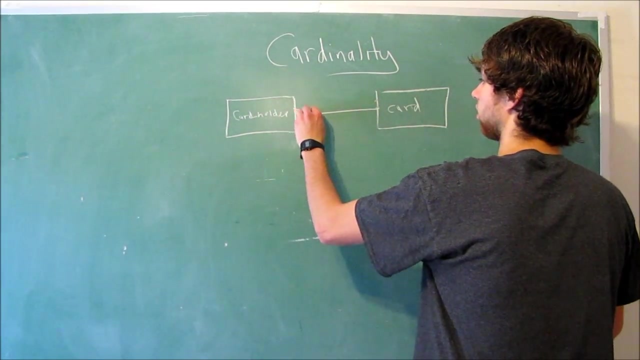 this guy has a lot of credit cards, So all of these rows can be connected to an individual row within the card holder table. Now let's look at it the other way. We could have a many-to-one relationship, or basically a one-to-many going the other direction, So we could have this. So now, 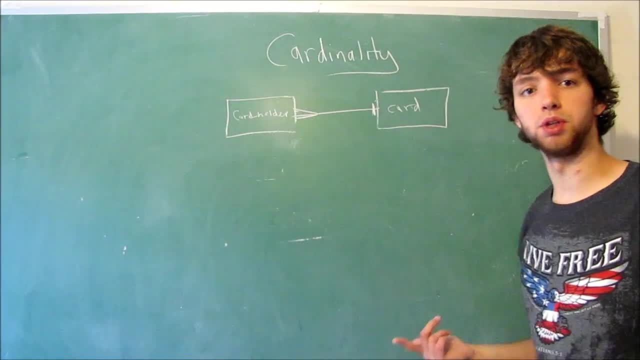 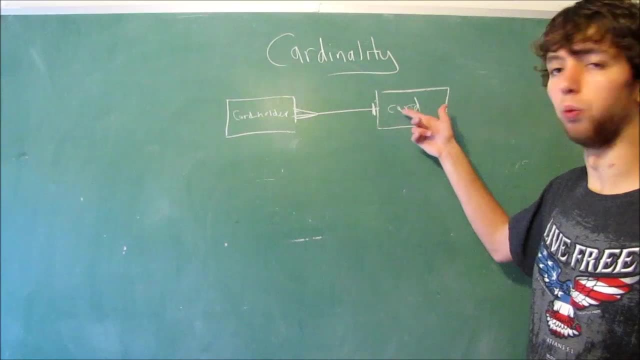 one card can be connected to multiple people, but multiple people can't be connected to one cardI'm sorryone card can be connected to multiple people, but they're not connected. So one card is not connected to multiple people, But one cardholder can only be connected to one card. 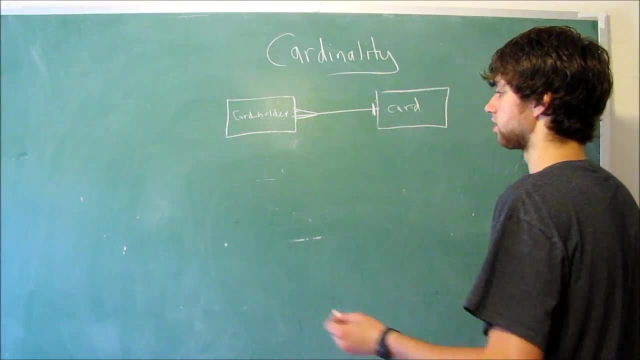 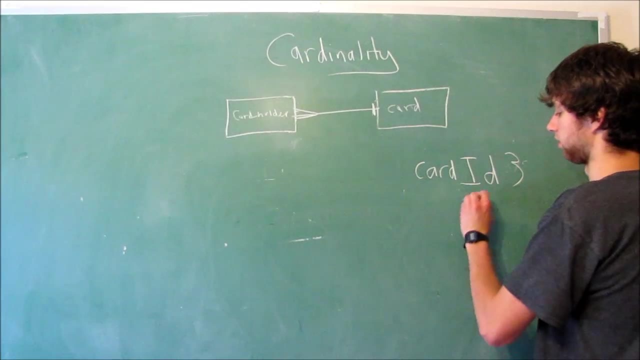 So that means one person cannot own more than one card. So now we think of it the other way around. We have a card with the ID 3.. We have a card with the ID 4. The ID of 6. It doesn't really matter what the numbers are. 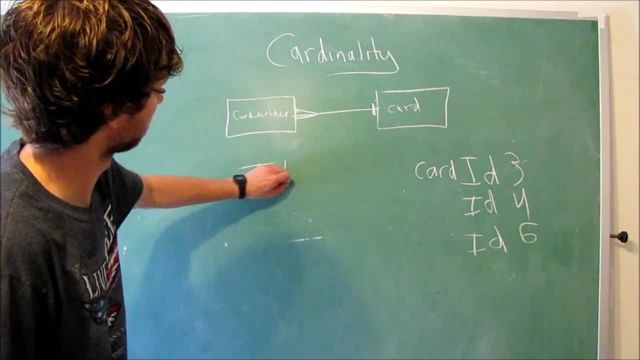 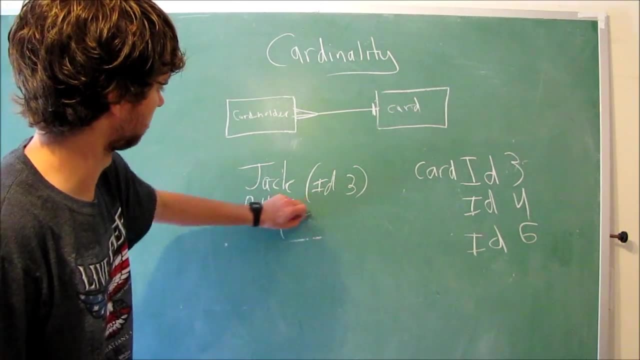 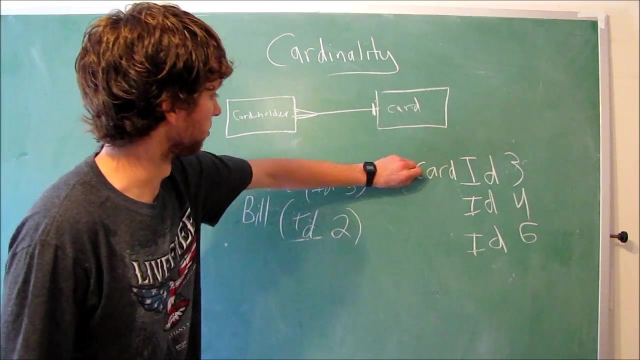 And then we have a cardholder. We just got a guy named Jack which ID is 3.. And then we got Bill ID of 2.. Well, we can have one card attached to many people, So this card could be attached to many people. 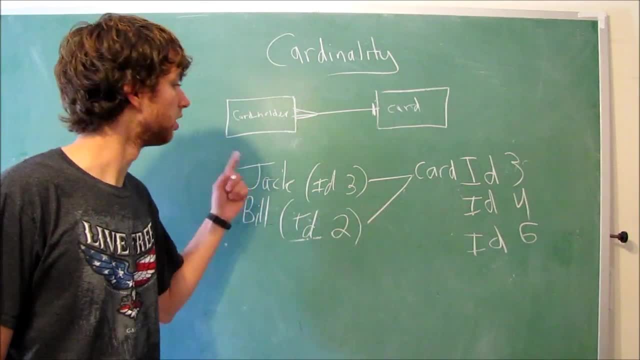 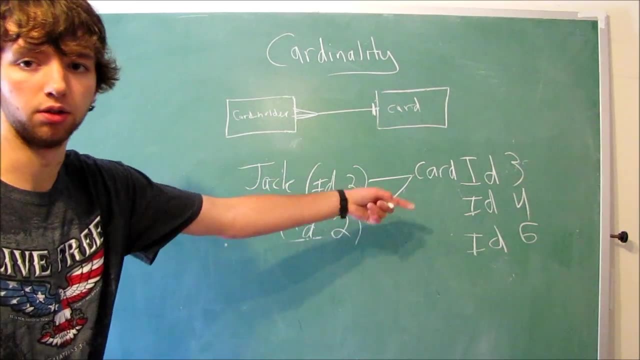 which means these people co-own a card. They're both the owner of one card. But now you have to realize an individual cardholder can't be connected to multiple cards, So Jack cannot own another card. That's not going to work out. 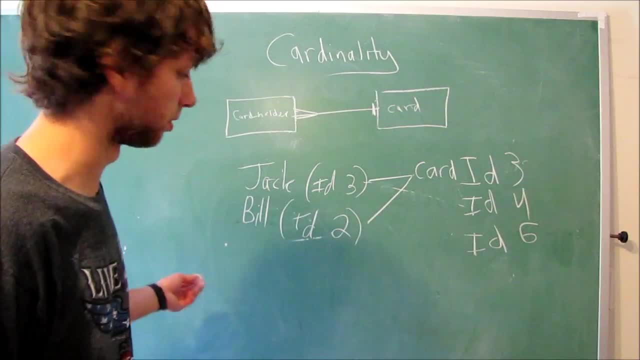 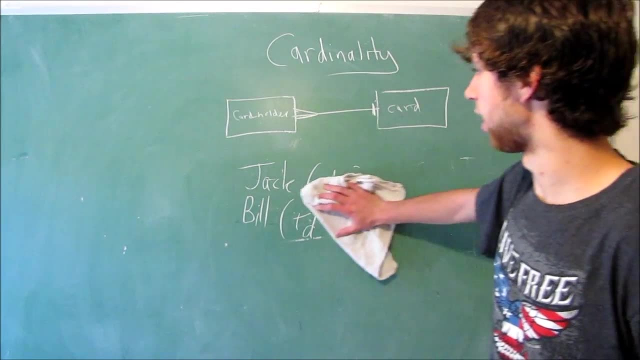 If you wanted that to work out, then you'd have to have a cardholder, You'd have to have the intermediary table which we talked about in designing many-to-many relationships, And this video is less to be a review of relationships but more of how to draw them.